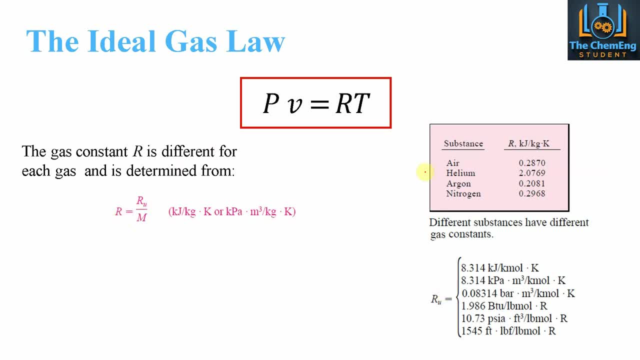 gas constant. R is the gas constant for the individual types of gases. So, in order to find the universal, we can rearrange this equation and we can have: RM equals RU. So therefore, if we have RU, ie the universal gas constant, we have the molecular mass. 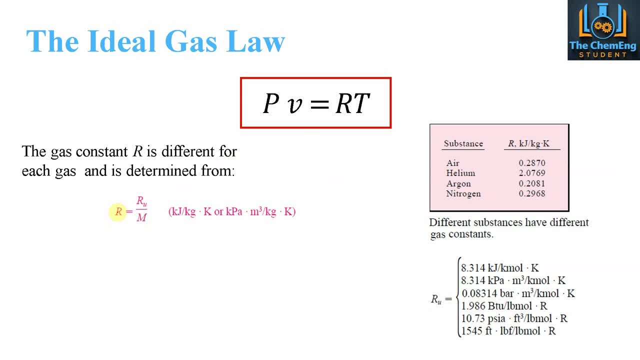 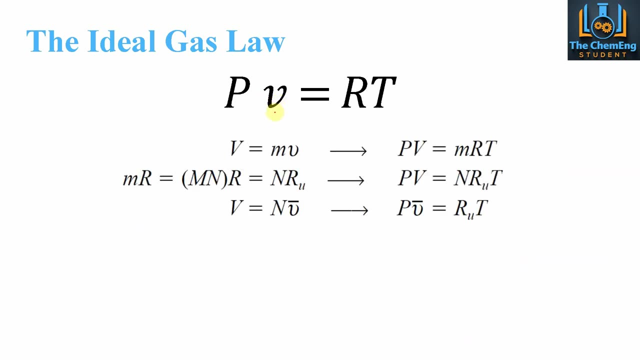 we can then calculate the gas constant for the specific substance. So again, that's just highlighting the different parameters here. Now, if we take the equation here, then what we can do is we can start to rearrange this for different purposes. So we start off with: 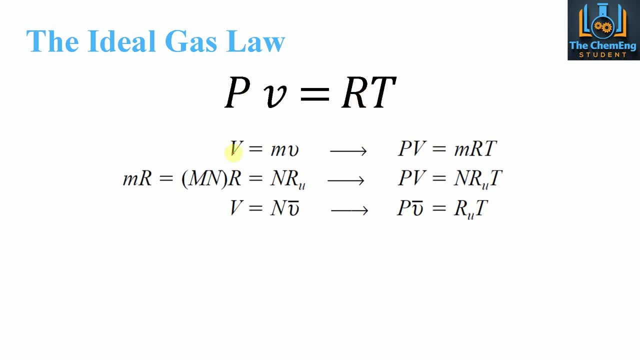 PV equals RT. So we start off with PV equals RT. Now, if we say that V equals RT, then we can start off with PV equals RT. So if we say that V is equal to M multiplied by V, then we can rearrange this to have PV equals MRT. This is one that is most familiar with chemical. 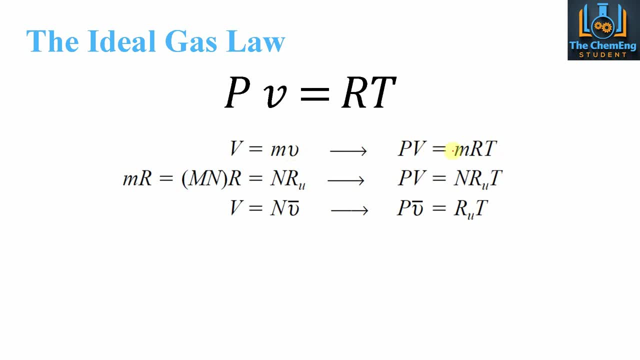 engineers. Now we can also simplify this and have: MR is equal to the MN multiplied by R, which can also be written as N, so that's the number of moles multiplied by the universal gas constant. So here we'd have: PV equals NRT. So again, this is another one that is commonly used. 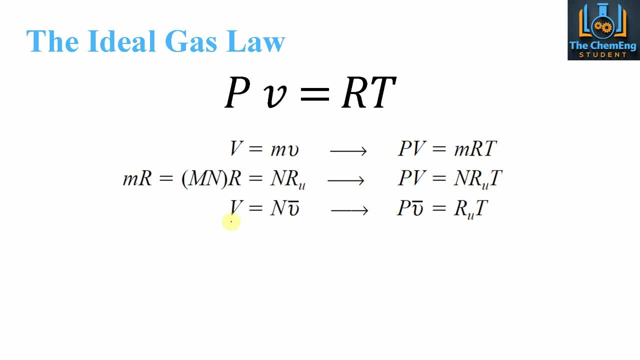 by chemical engineers- One that is not so common- is: V equals the number of moles multiplied by the average specific volume of the material. Now what we would therefore do is we can replace the V here with N and V bar, And then what would happen is the Ns would count as the number of moles multiplied by. 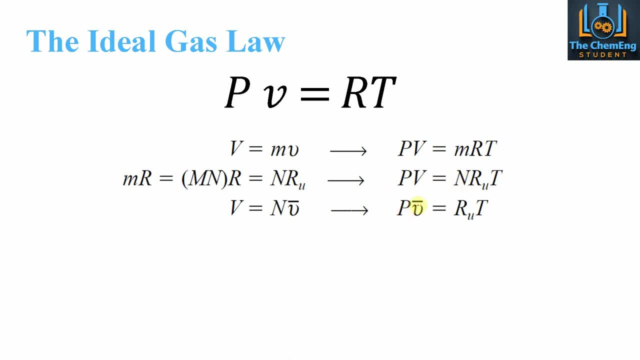 the average specific volume of the material. Now, what we would therefore do is we can replace the V here with NRT, so that we'll have PV equals R, and then we can have PV equals RT multiplied by V. We now move on to the next part of our small section of the program. We're left with 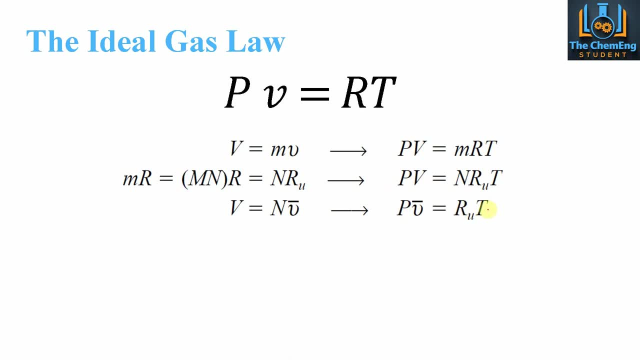 P V bar is equal to the universal gas constant multiplied by the temperature. So depending on the information that we have, we can use and manipulate this equation to suit our system. And again there we have all the different parameters here. So again you can just take. 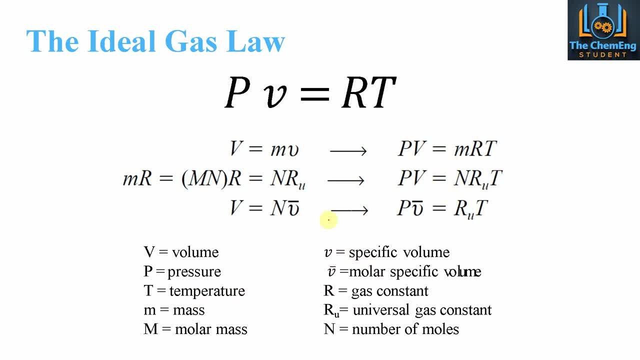 a look at these and see if you can derive these equations again by yourself. But again, if you have problem with this, you can have the same returned for the other equations have problems? you can always refer back to this slide for some help. Now the ideal gas equation. 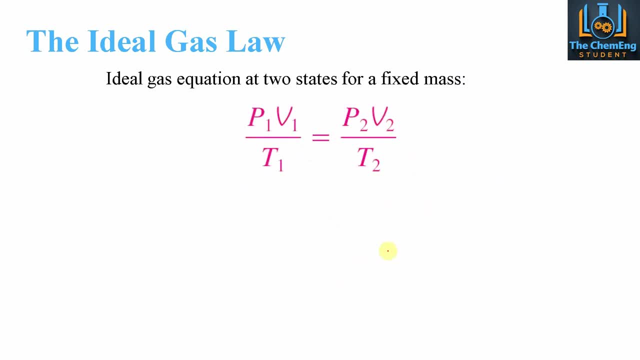 at two states, for a fixed mass can be given by this expression here. So we have p1: v1 over t1 is equal to p2, v2 over t2.. So this is the relationship for the equations of state Now we'll look at all the different types in just a second. Now, when we have these types of systems, 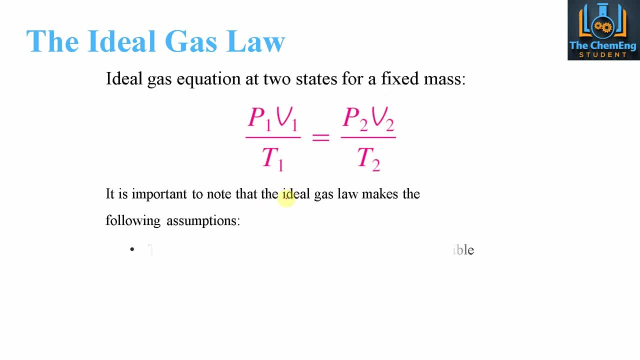 it is important to note that the ideal gas law makes the following set of assumptions That we have. the volume occupied by the gas molecules is negligible compared to the overall system and it neglects the interaction forces between the molecules themselves. If we have any deviations, 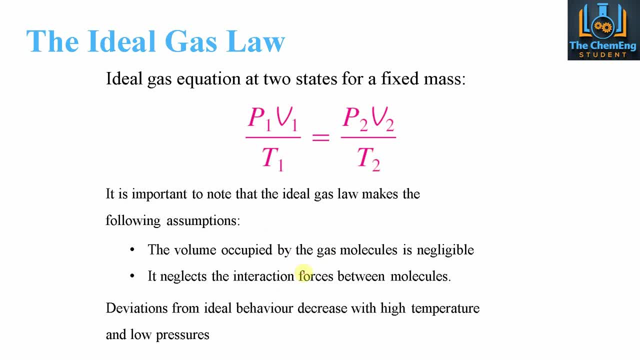 from this behavior then, with how we do it, we can get the same result. So if we have any deviations, higher temperatures and lower pressures- we cannot assume ideal gas conditions. We would therefore have another type of equations that we would have to solve, and we look at how to solve non-ideal gas. 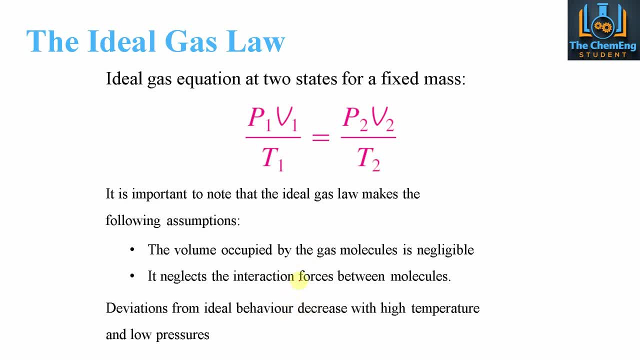 systems in our thermodynamics course. So if you want to know more about that, I'll put a link in the description to our thermodynamics course and you can take a look at that in your spare time. Now the equations of state we have set up in the previous slide for a fixed mass equation. So we have p1, v1 over t2 over t2 over t2. 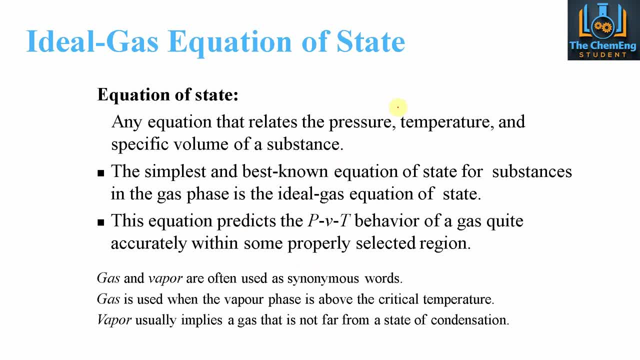 and we have several different types that we'll look at here so that you are familiar with all the different types, so that, depending on the question and the information provided, you will be able to solve, regardless of the type of information that you have. So here, any equation that relates the 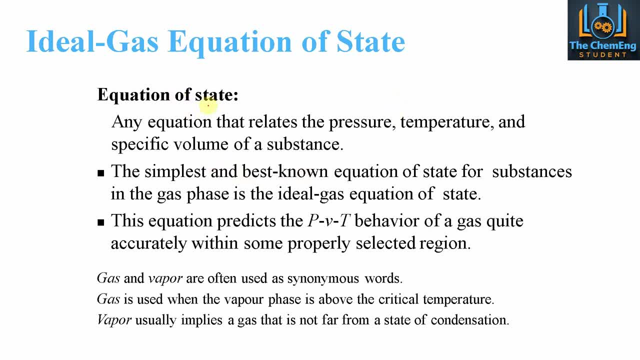 pressure, the temperature and the specific volume is for the equation of state. Now, this is in terms of the gas phase, is for ideal gas equations of state. So if we have any deviations from the state and the equation predicts the p v, t behavior. so that is the pressure of the specific volume. 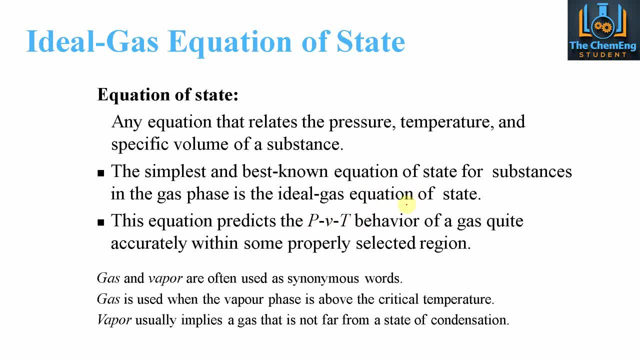 and the temperature of a gas, which is fairly accurate. Now, a gas and vapor are often used as synonymous words, whereas the gas is, the vapor phase is above the critical temperature, and vapor implies a gas that is not far from its state of condensation. So that's just a couple of. 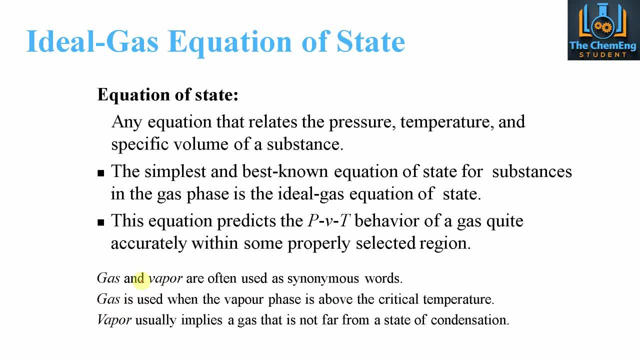 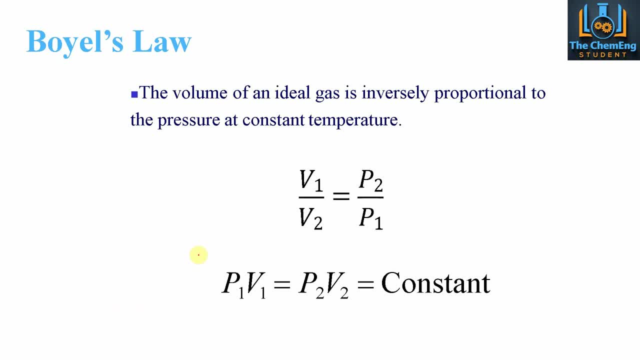 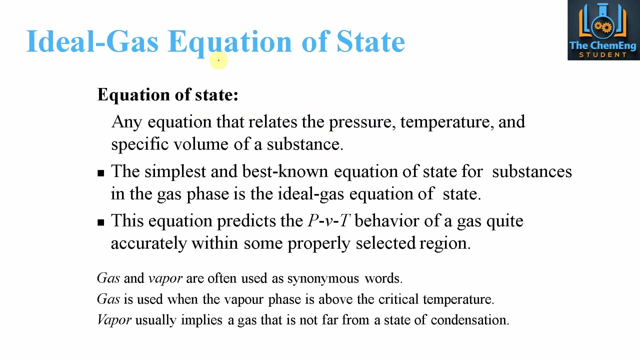 points to note As we go through this, that if we refer to gas and we refer to vapor, that we can distinguish the two. So the first one here is Boyle's law. Now Boyle's law has the ratio between the volume and the pressure. So what we have fixed here is the temperature. So from this equation here, this is: 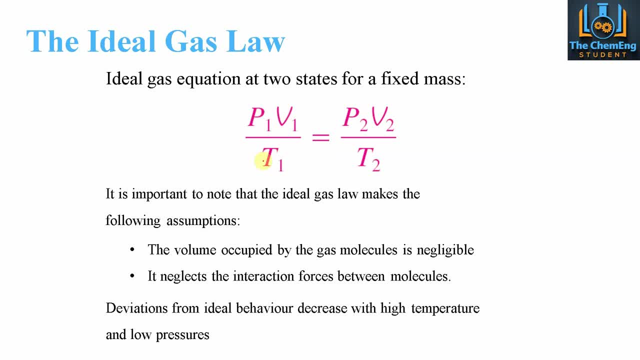 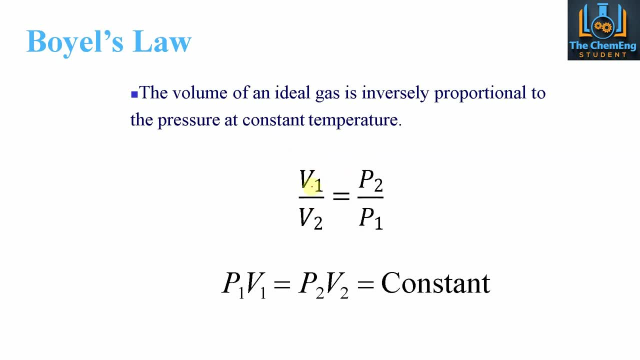 what we're going to manipulate between the pressures, the specific volume and the temperatures. So, by fixing the temperature, what we have is the ratio of the volumes v1 over v2 is equal to the ratio of p2 over p1. Now, when we cross, multiply these, we get p1, v1 is equal to p2, v2 and that 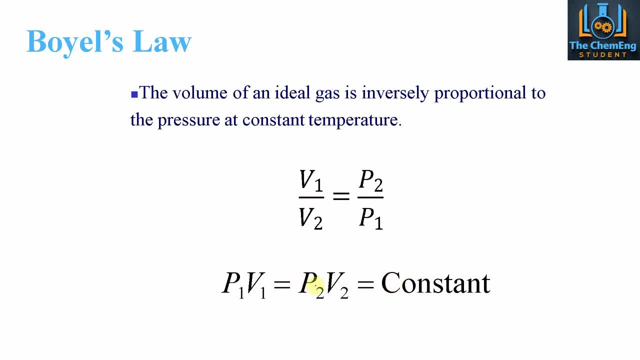 would equal some form of constant. So where this becomes useful is if we fix the temperature of our system, if we know the properties at, say, point one and we know the pressure at point two, So when we cross from that we can then calculate the value of v2. and that's where these equations 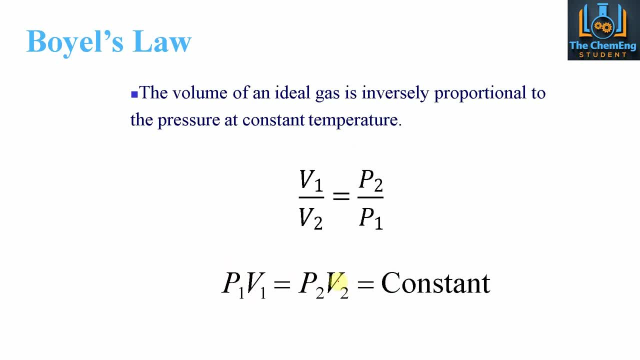 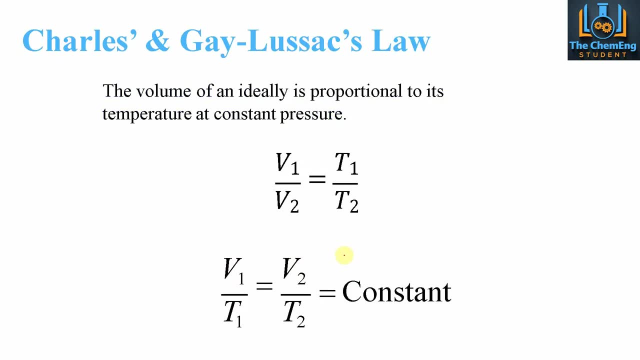 of state can be very useful. If we fix one of the variables, we can therefore find the unknown values. Now we have the Charles law, which is when we fix the pressures this time. So by fixing the pressures, we have the relationship v1 over v2 is equal to t1 over t2.. Again, that's manipulating the 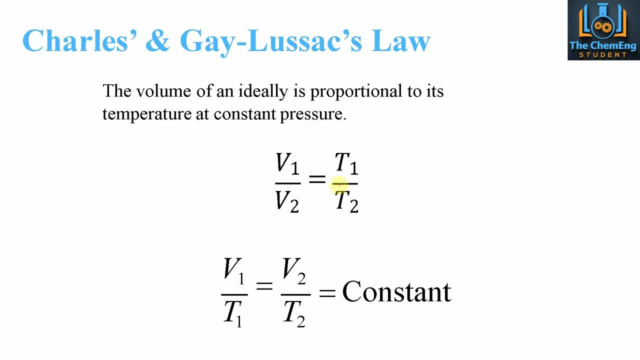 equation that we've seen earlier. So we can now create a equation that's going to be equal to t1 over t2.. the beginning of the equations of state. So when we cross, multiply these- if we needed to- we would have t2 v1 equals t1- v2.. So because we mix the twos and the,